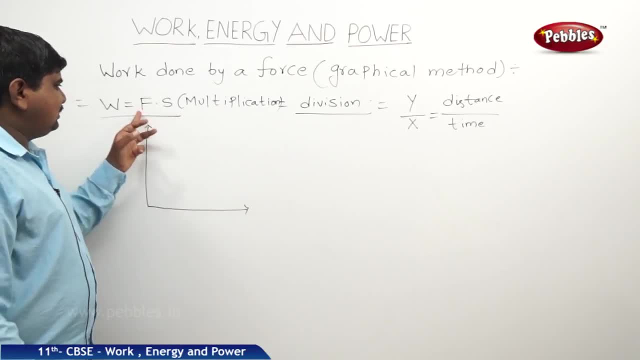 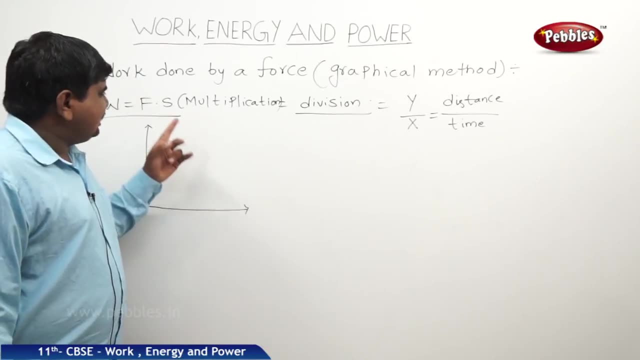 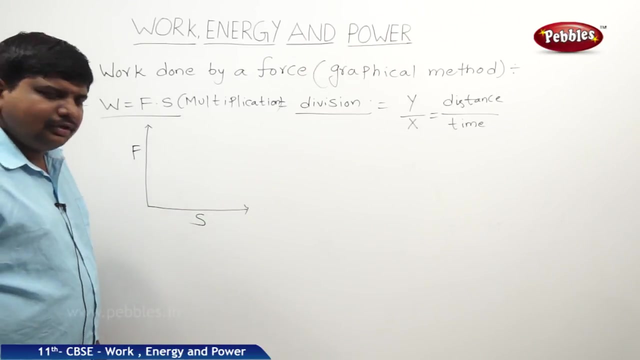 is a result of multiplication of two physical quantities, such like force and distance. in this case, there is no rule like this. you can take f on x or y axis as well as distance on x or y axis, so we can take f, yes, so if this is the graph, if the work done is uniform, for one newton of the 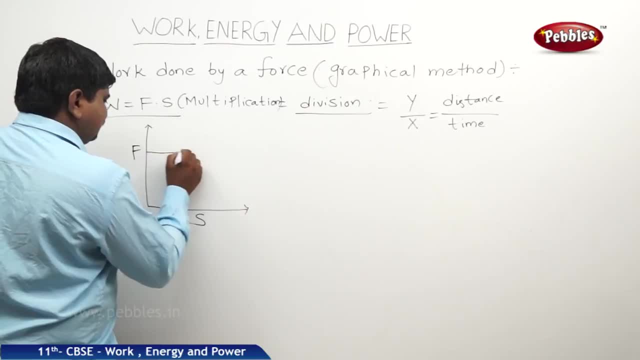 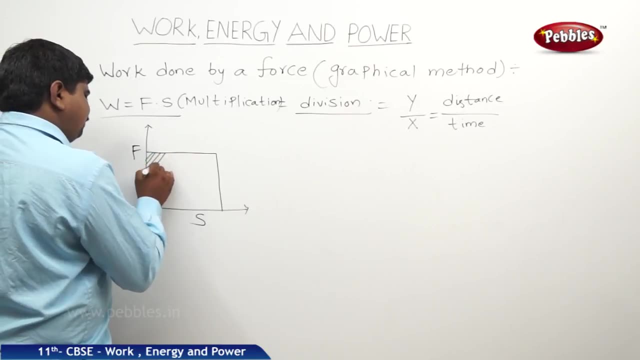 force and one meter of the displacement, you will get a graph like this: so this is area occupied by the shade of the graph. let us suppose if this area occupied by the graph or the shade of the graph occupies any rectangular shape or square shape like this, we can take the area of that particular geometrical shape. then 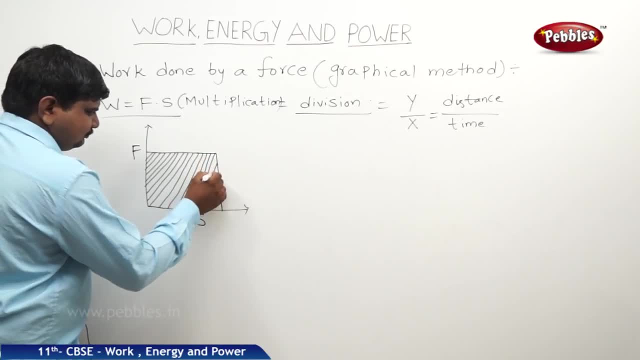 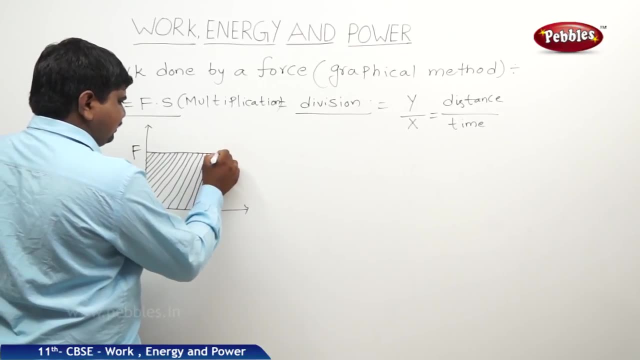 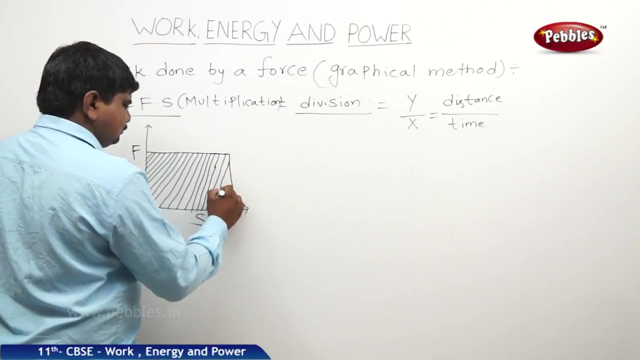 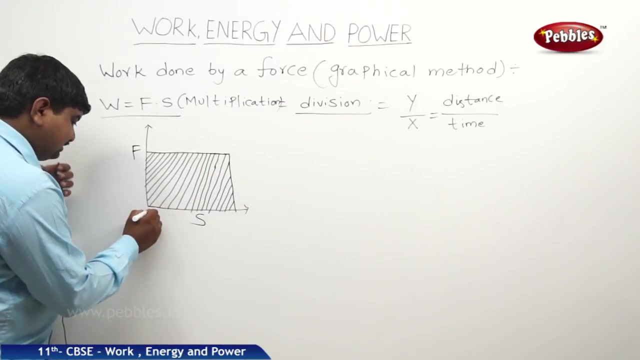 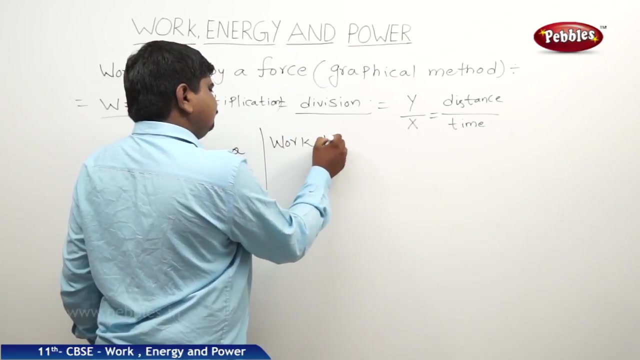 that will give the work done by the body. so as well as, let us suppose if this occupied some rectangular shape. so let us suppose the origin is o, this is p, this is q, this is r. in this case, if the graph is shaped like this, work done is equal to area of the graph. 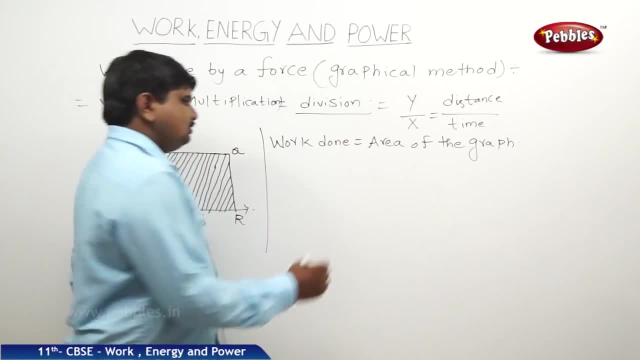 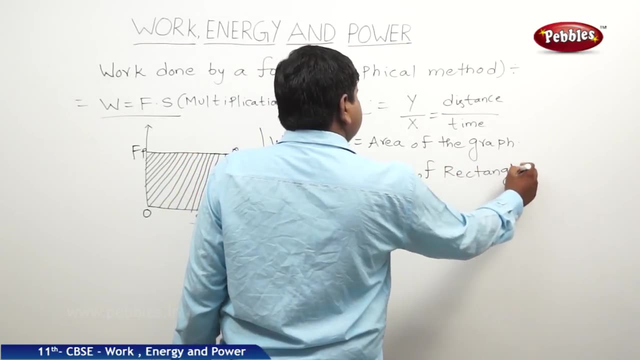 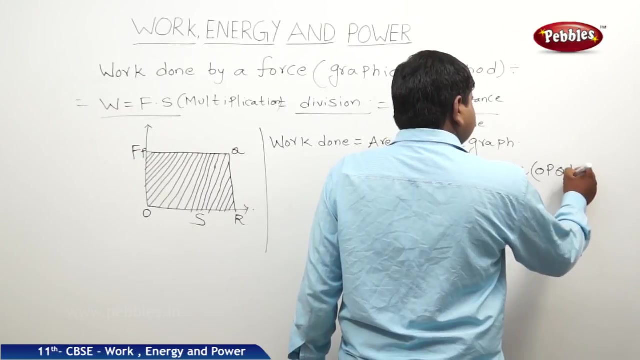 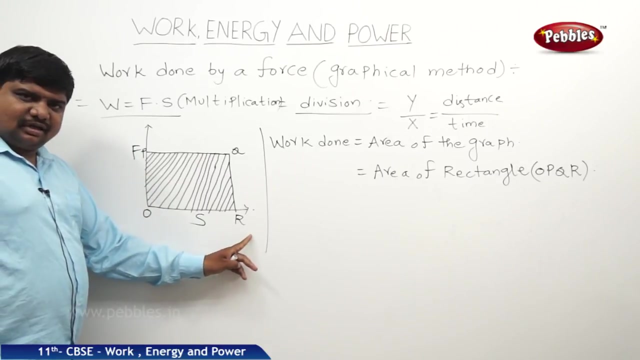 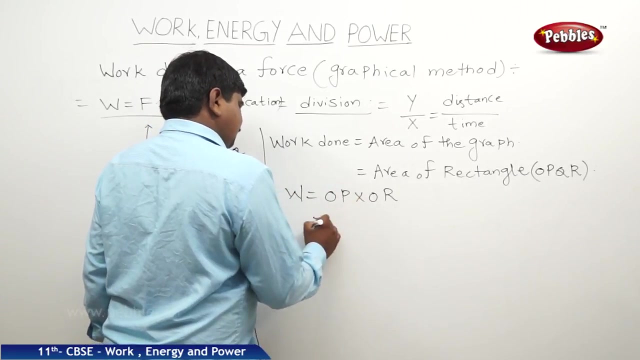 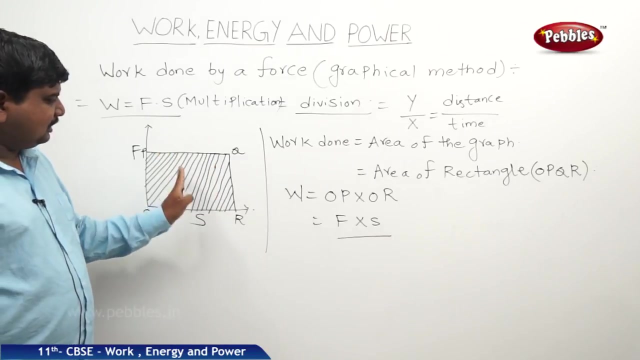 now the graph is in a rectangular shape, so it will become area of rectangle. the name of the rectangle is op. qr force represents this column, op s represents this column, or therefore w is equal to op. into where, where op represents f, where or represents s. such like this, we can draw the graph and we can derive the relationship between the. 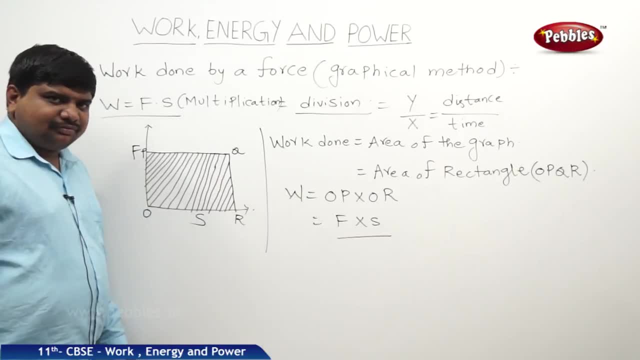 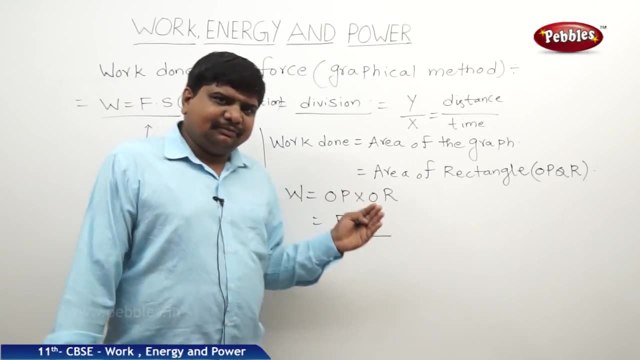 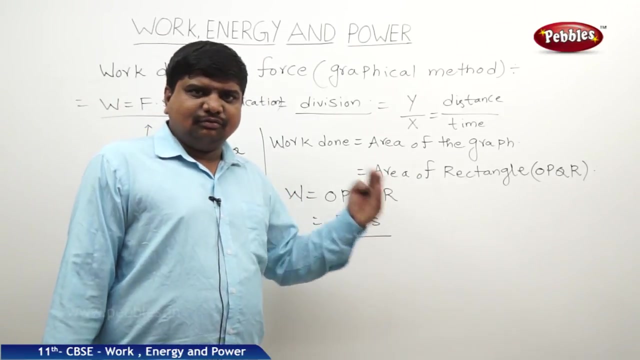 work between force and displacement. with respect to the graph, this is the graph for a force which is applied for single time means a constant force. if the force is variable, there may be a chance for the change in the shape of the graph. this case is called work done by a variable force. we will check now. now we will see that the 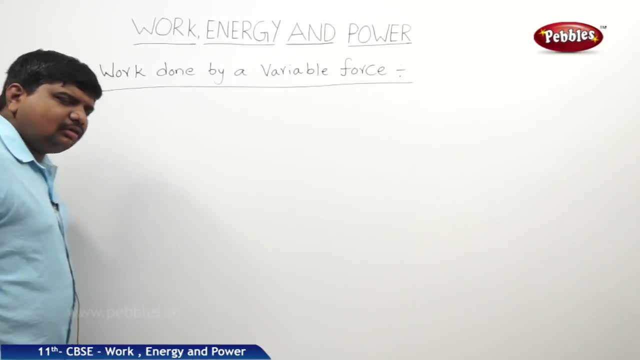 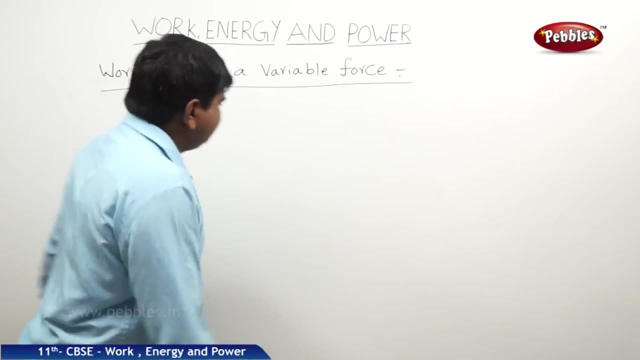 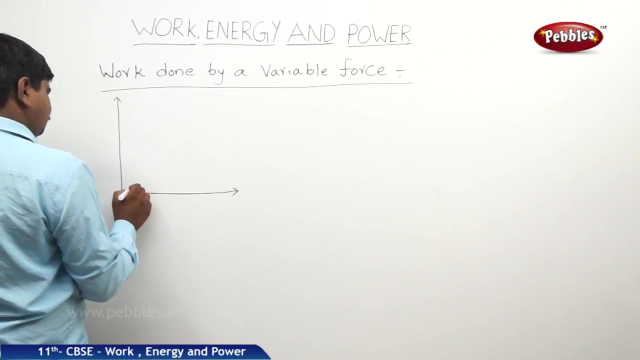 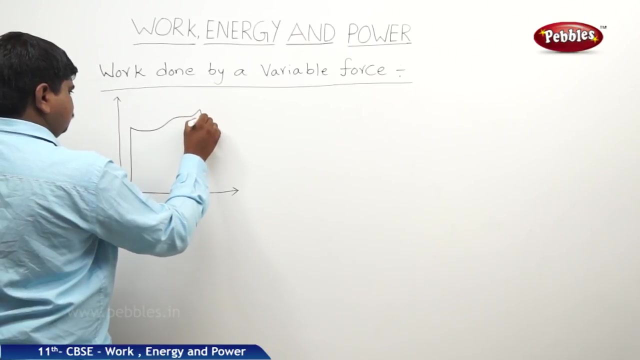 work done by a variable force. That means force is not constant Once it is not applied and it is constant throughout the motion. it is not like that Force is continuously changing. So for that case, this might be the graph. So, along this direction, this: 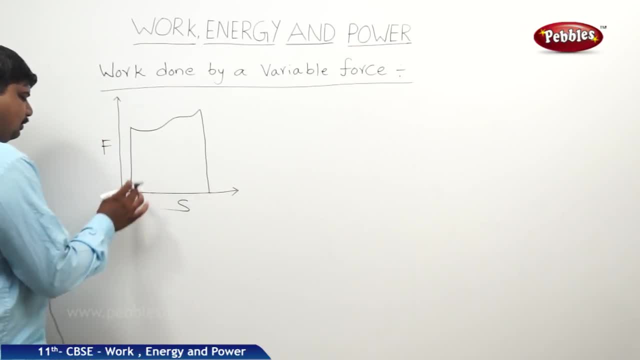 is F, this is S, So the body was moved from one point to another point. So in this point it was under the variation of the force, or it is applied to the variable force In this variation. let us take a small variation: This is P, this is Q, this is R and this is S, Where PQ is. 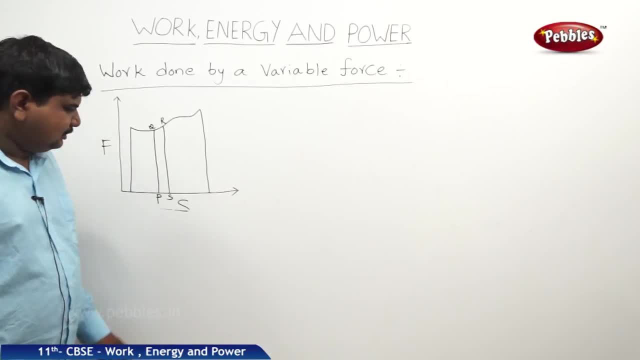 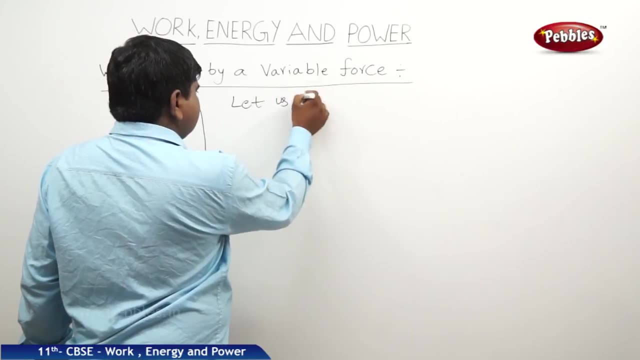 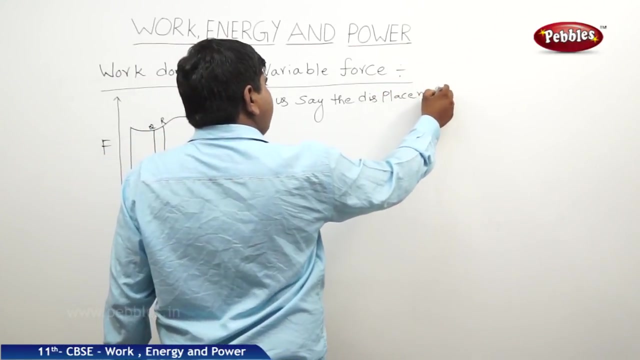 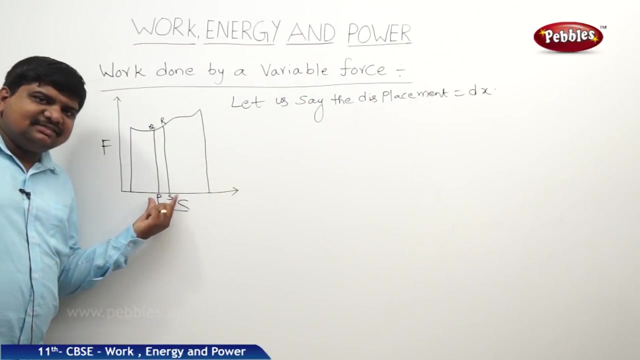 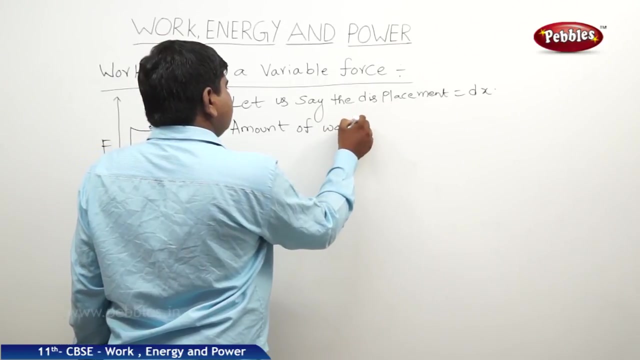 in the direction of force, where PS is in the direction of S. So this PS is the small displacement. Let us say the displacement is dx, So this is Q, So the amount of work done in moving this small distance will be dW In. 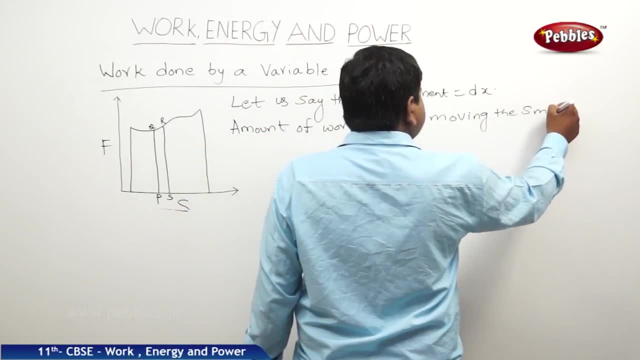 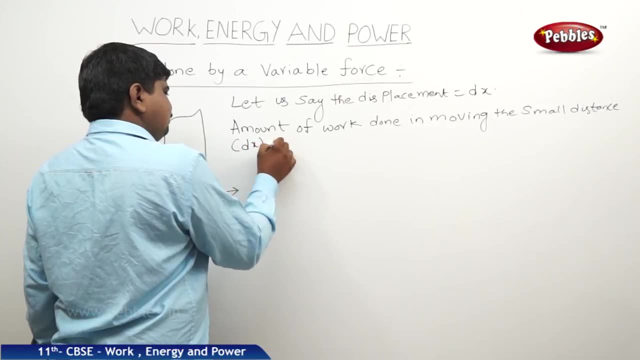 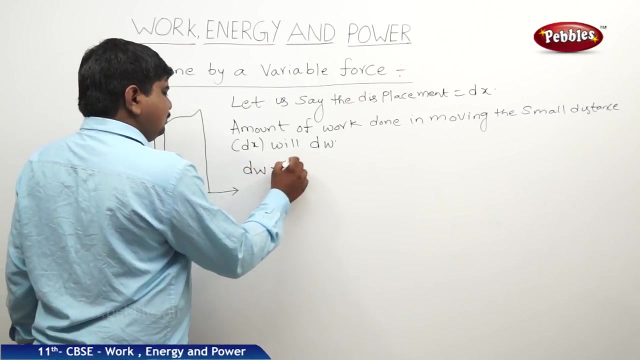 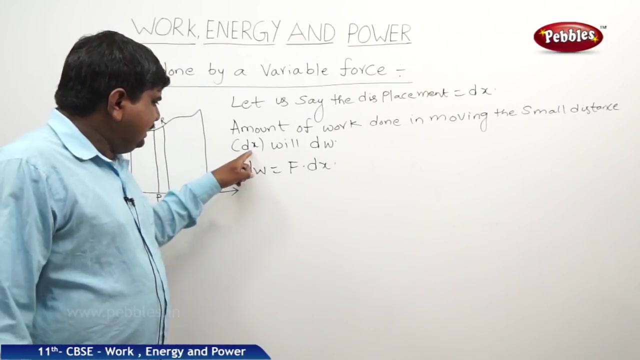 moving the small distance, dx will be dw, So therefore dw is equal to f dot dx. So total work done will be integrating. 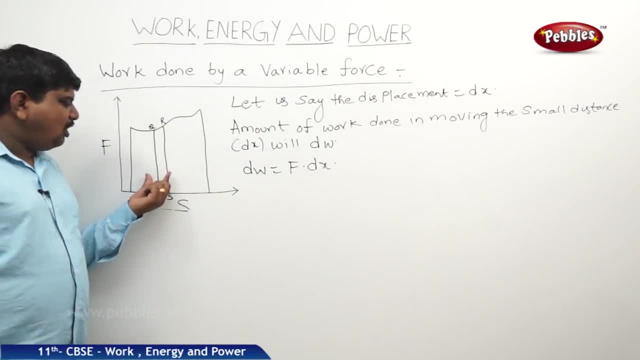 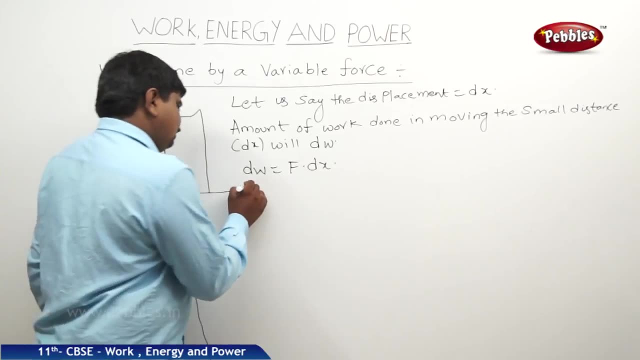 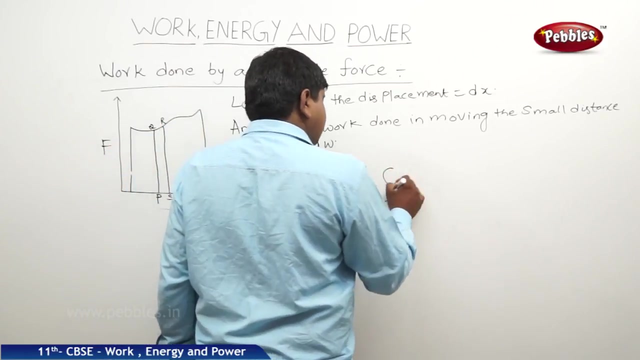 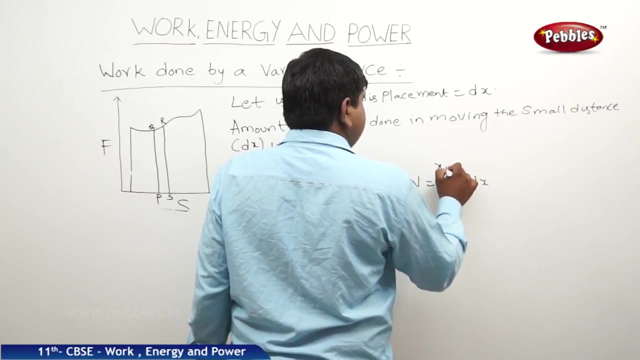 on both sides, where differentiation is taking a small element from a big one, where integration is extending the small one to the bigger one. So total work done is equal to integral dw, is equal to integral f, dot, dx, where positions are xa to xb. So the differentiation and